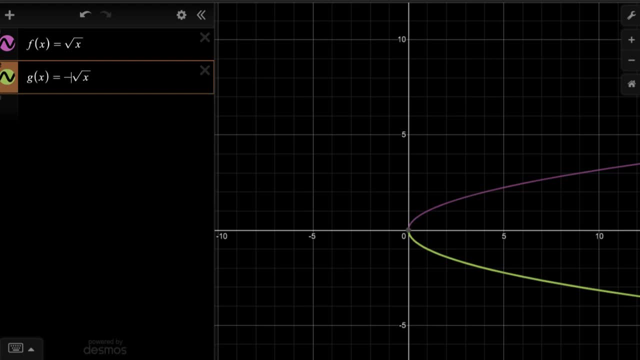 It looks like it reflected it over the x-axis. Now, instead of doing it that way, what if we had another function, h of x? and I'll start off by making it identical to f of x? So once again, it's right over there. 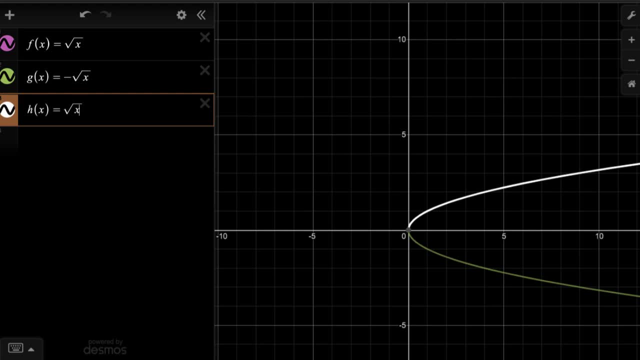 It traces out f of x. Instead of putting the negative out in front of the radical sign. what if we put it under the radical sign? What if we replaced x with a negative x? What do you think is going to happen there? Well, let's try it out. 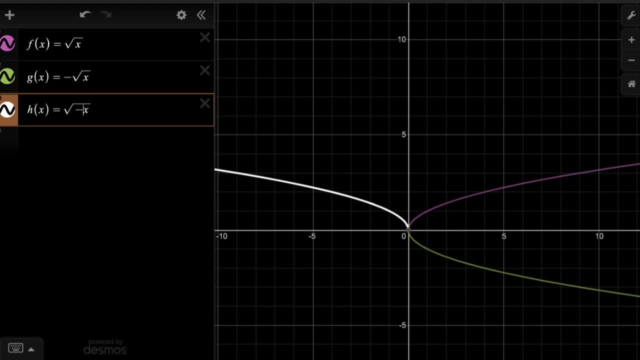 If we replace it, that shifted it over the y-axis And then pause this video and think about how would you shift it over both axes? Well, we could do a. well, I'm running out of letters, Maybe I will do a, I don't know. k of x is equal to. 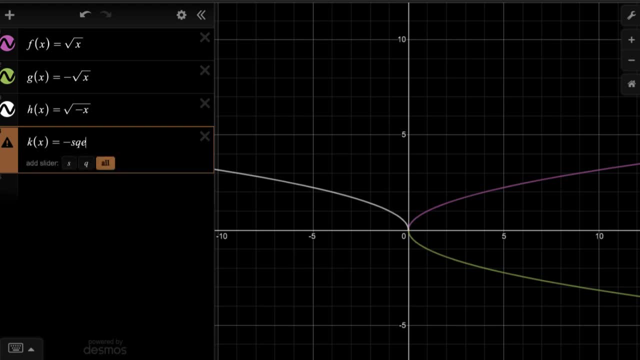 so I'm gonna put the negative outside the radical sign and then I'm gonna take the square root and then I'm gonna put a negative inside the radical sign And notice it flipped it over both. It flipped it over both the x-axis and the y-axis. 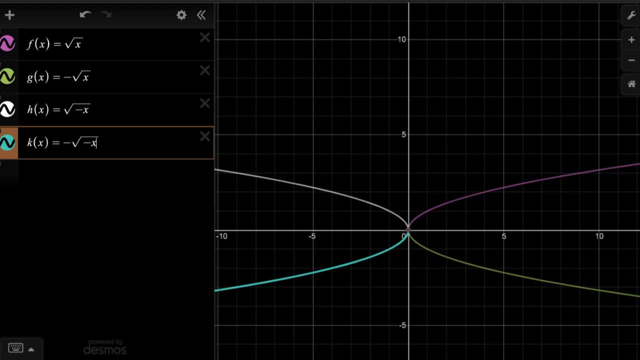 to go over here. Now, why does this happen? Well, let's just start with the g of x. So when you put the negative out in front, when you negate everything that's in the expression that defines a function, whatever value you would've gotten of the function before, 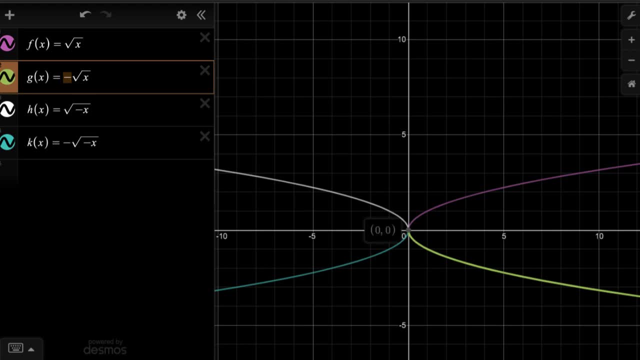 you're now going to get the opposite of it. So when x is zero, we got zero. When x is one instead of one, now you're taking the negative of it. so you're gonna get negative one When x is four instead of getting positive two. 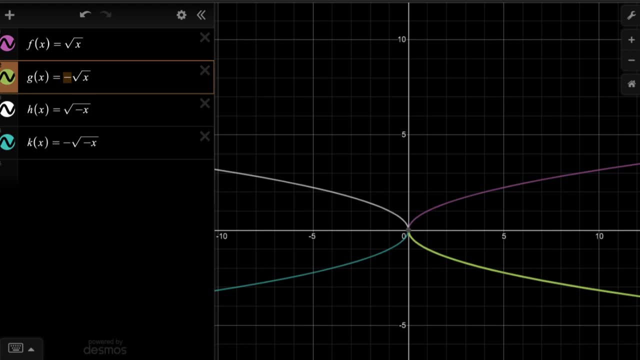 you're now going to get negative two When x is equal to nine. instead of getting positive three, you now get negative three. So hopefully that makes sense. why putting a negative out front of an entire expression is going to flip it over. flip its graph over the x-axis. 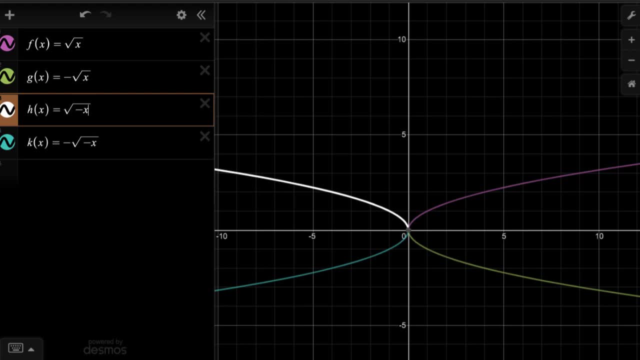 Now, what about replacing an x with a negative x? Well, one way to think about it now is, whenever you inputted one before, that would now be a negative one that you're trying to evaluate the principal root of, And we know that the principal root function. 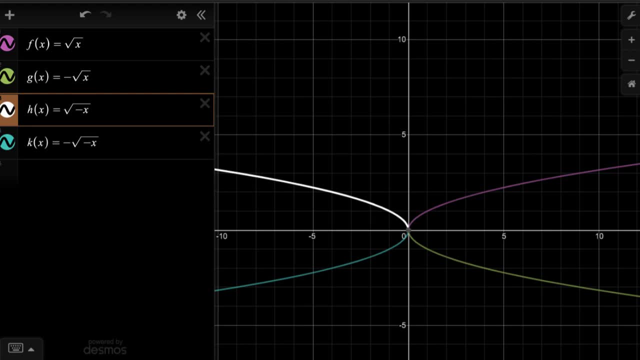 is not defined for negative one, But when x is equal to negative one. our original function wasn't defined there, when x is equal to negative one. But if you take the negative of that, well, now you're taking the principal root of one. 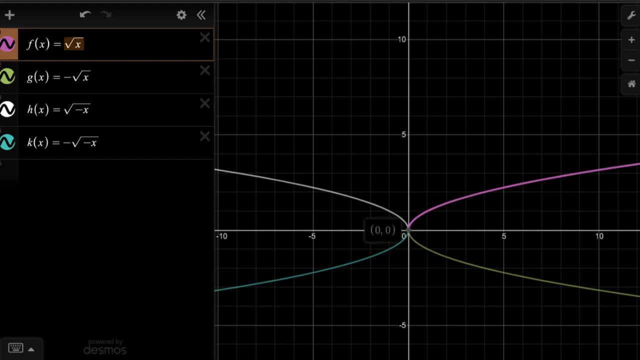 And so that's why it is now defined. So, whatever value the function would've taken on at a given value of x, it now takes that value on the corresponding opposite value of x and on the negative value of that x, And so that's why it flips it over. 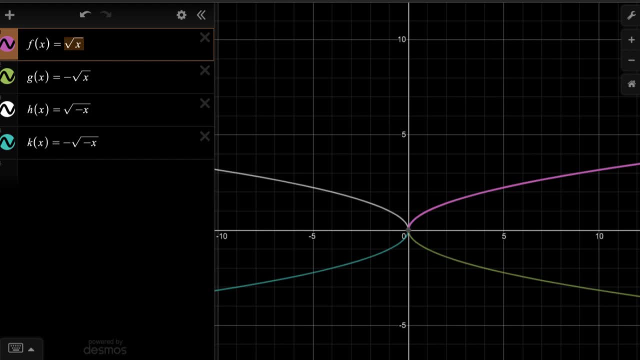 and it flips it over to the x-axis. And this is true with many types of functions. We don't have to do this just with a square root function. Let's try another function. Let's say we tried this for e to the x power. 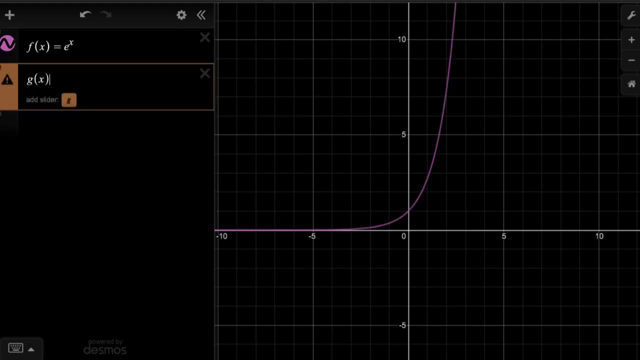 So there you go. we have a very classic exponential there. Now let's say that g of x is equal to negative, e to the x, And if what we expect to happen happens, this will flip it over the x-axis. So let's say that g of x is equal to negative e to the x power. 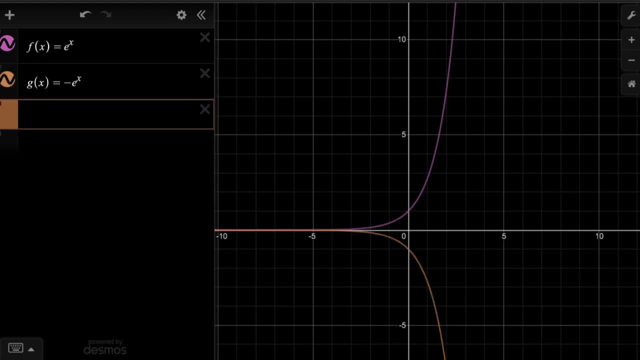 And indeed that is what happens. And then how would we flip it over the y-axis? Well, let's do an h of x That's going to be equal to e to the. instead of putting an x there, we will put a negative x, negative x. 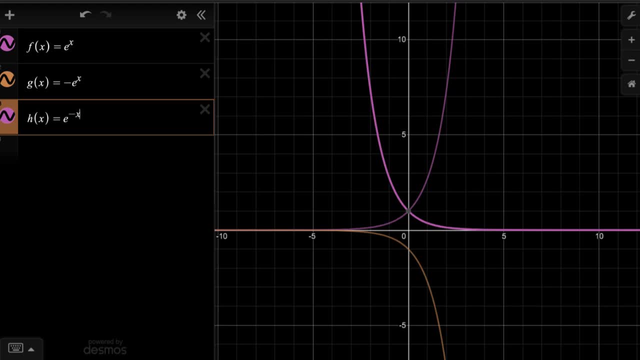 And there you have it. Notice it flipped it over the y-axis. Now, both examples that I just did, these are very simple expressions. They're complex. Let's say that f of x. let's give it a nice higher degree polynomial. 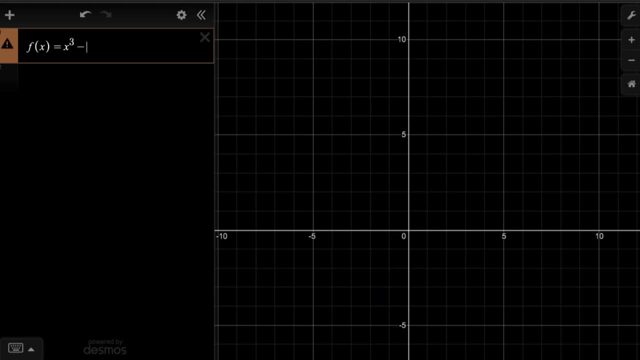 So let's say it's x to the third minus two x squared. That's a nice one, And actually let's just add another term here, So plus two x. Oh no, I want to make it minus two x. I want to accentuate some of those curves. 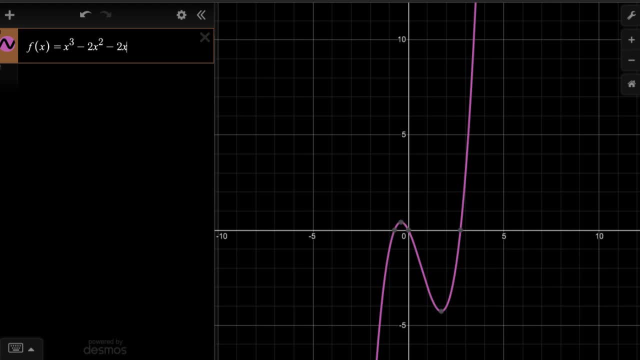 All right, so that's a pretty interesting graph. Now how would I flip it over the x-axis? The way that I would do that is: I could define a g of x. I could do it two ways. I could say: g of x is equal to the negative of f of x. 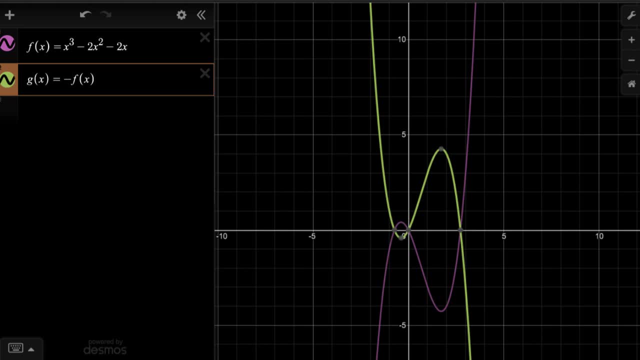 and we get that. So that's essentially just taking this entire expression and multiplying it by a negative one. And notice, it's multiplying it, it's flipping it over the x-axis. Another way we could have done it is: instead of that, we could have said the negative of. 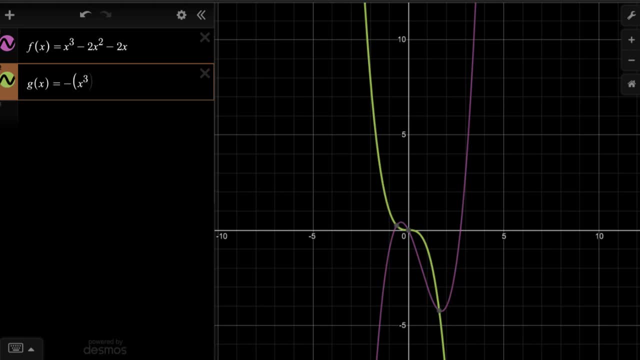 x to the third, minus two x squared, and then minus two x, and then we close those parentheses and we get the same effect. Now, what if we wanted to flip it over the y-axis? Well then, instead of putting a negative, 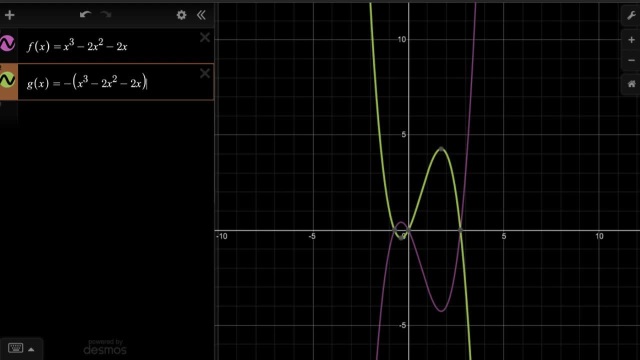 on the entire expression. what we want to do is replace our x's with a negative x. So you could do it like this: You could say that that's going to be f of negative x and that has the effect of everywhere. you saw an x before. 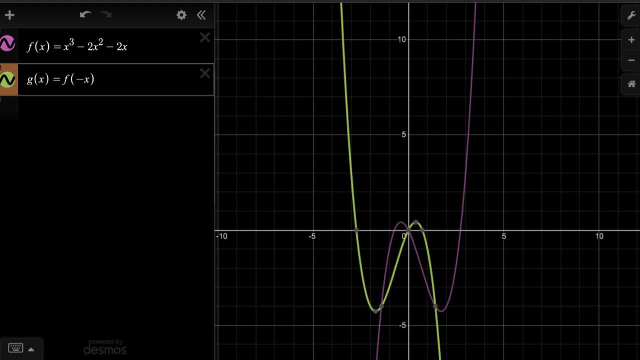 you replace it with a negative x And notice it did exactly what we expect: It flipped it over over the y-axis. Now, the other way we could have done that just to make it clear. that's the same thing as negative x to the third power. 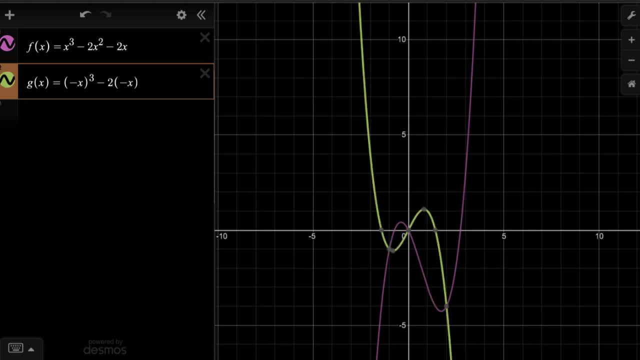 minus two times negative x, squared minus two times negative x, And of course we could simplify that expression. but notice it has the exact same idea. And if we wanted to flip it over both the x and y-axis, well, we've already flipped it over the y-axis. 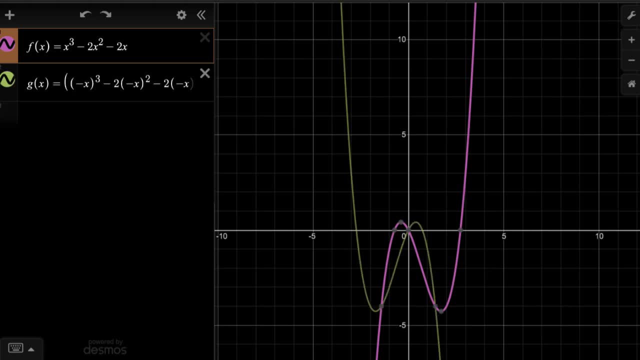 To flip it over the x-axis. whoops, I just deleted it. To flip it over the? I'm having issues here. To flip it over the x-axis as well. we would. oh, they gave me a parentheses already. I would just put a negative out front. 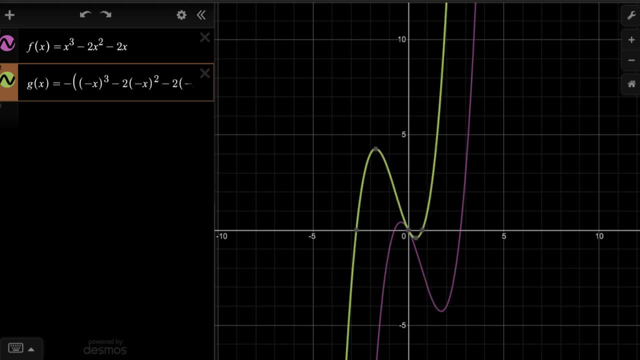 So I put a negative out front and there you have it. This flipped it over both the x and y-axis. You can do them in either order and you will get to this green curve. Now, an easier way of writing. that would have been just. 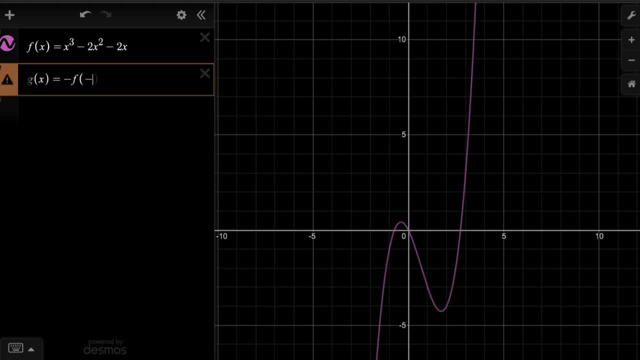 the negative of f, of negative x, and you would have gotten to that same place. So go to Desmos, play around with it. Really good to build this intuition and really understand why it's happening.